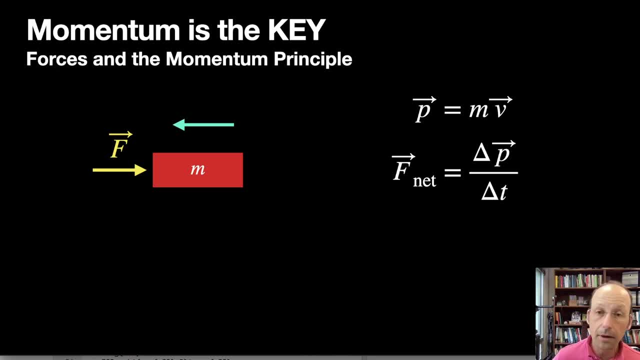 force. I could write that as the change in momentum divided by the change in time. But if it's not, that's fine too. So imagine how that would work. Here's some object moving with the momentum. P1 is actually moving to the left and a little bit later. I know I put. 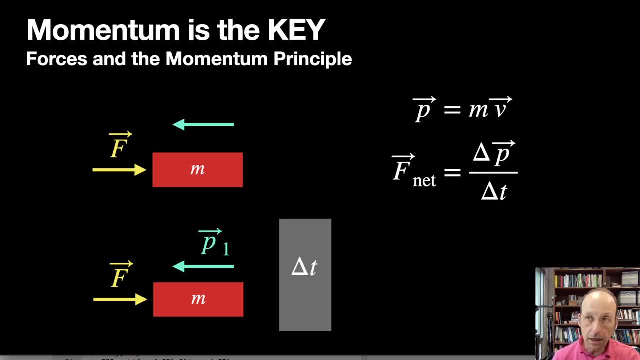 it to the right, there's a force pushing on it. So a little bit later, after some time interval- delta t- it has a new momentum, P2.. That change in momentum, P2 minus P1, is dependent on the force. And, yes, it depends on the mass, because the momentum depends on the mass. 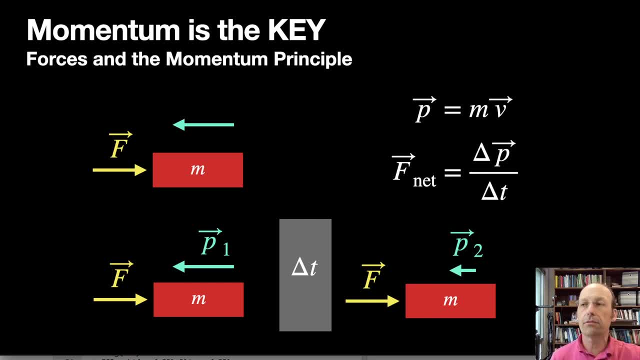 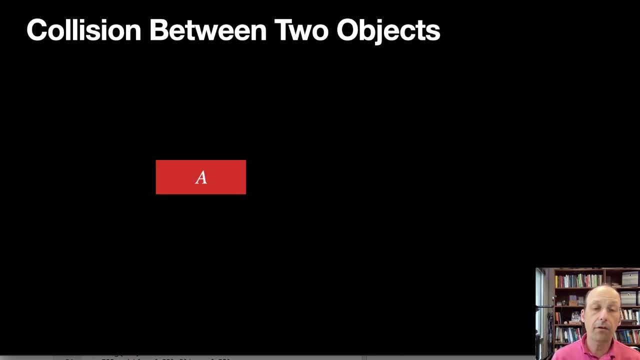 This is technically the same as Newton's second law, but it just just hold on. just work with me here, Okay. So what about collisions between two objects? Suppose I have some object I'm called mass A and then it is moving and it collides, it comes in contact with mass B. What happens? 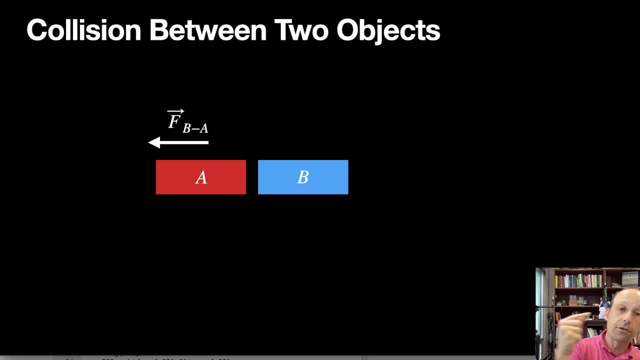 Well, first of all, there's a force that B exerts on A- And I'm going to write this as a vector force: B dash A, So it's the force that B pushes on A. Well, but it's a contact. 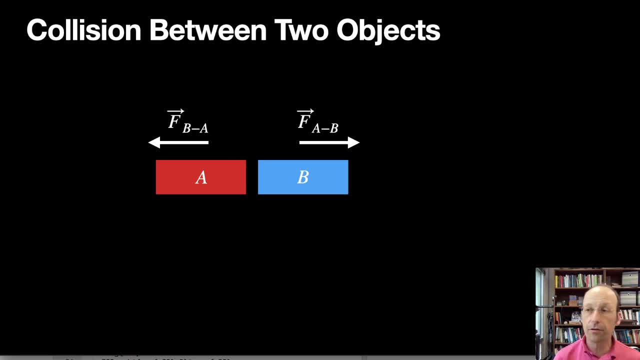 so actually A also pushes on B in the opposite direction. That's what happens. Forces are an interaction between two objects, so they both exert a force on each other. Let's look at car A and use the momentum principle. So the momentum principle says that the force on A 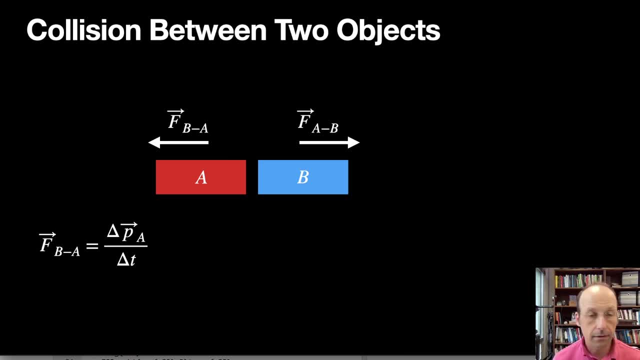 is the rate of change of momentum for object A, And then we could do the same thing for car B. The force on B is the delta P B divided by delta T. But those forces, FB on A and FA on B, are equal and opposite. 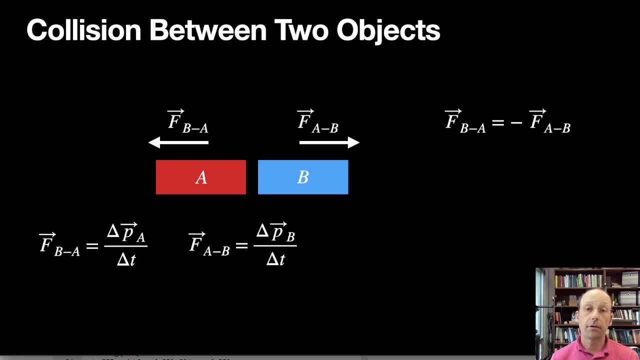 That's what's true for interactions. Forces come in pairs, So FBA is the exact opposite of FAB. Then that means there's a relationship between the changes in momentum. I can just say this: If they have the same time interval. 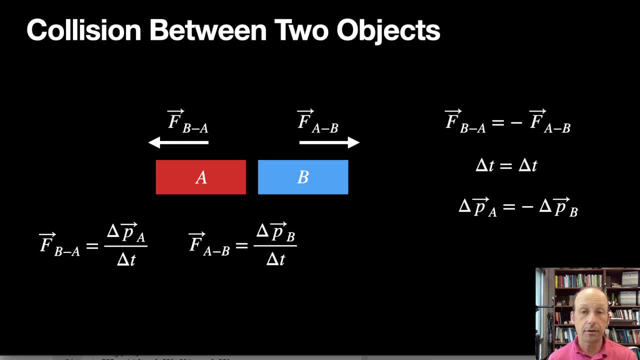 then their changes in momentum have to be equal and opposite. So the change in momentum for A has to be the exact opposite of the change in momentum of B, because the force on B is equal and opposite. So the forces are equal and opposite. If you want, you can move that momentum B to the other side. 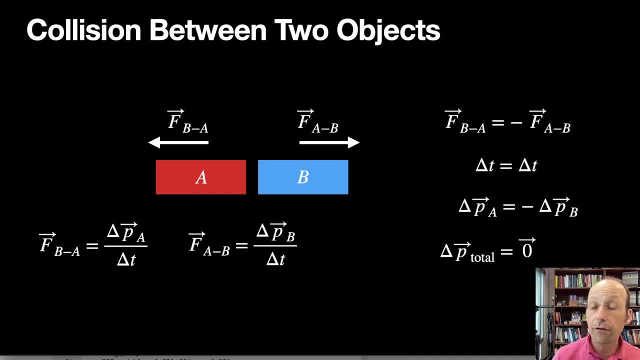 and just write it as the change in total momentum is zero. Or, if you want, you could write it as this: PA1,, which is the momentum of A before the collision, plus BB1,, which is the momentum of B before the collision. 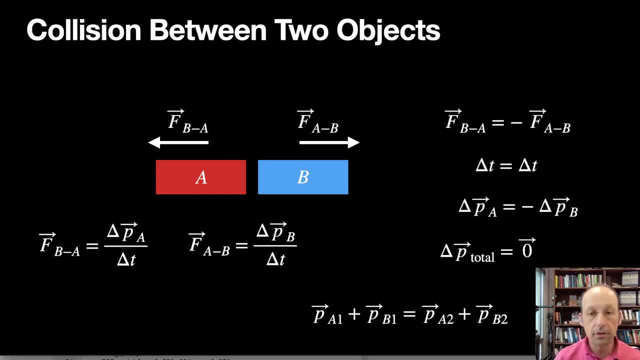 has to be equal to the momentum after, PA2, which is after, and PB2, after. So the momentum before is equal to the momentum afterwards. Afterwards- And we call this conservation momentum, because momentum does not change over the interaction. It's the same before as it was afterwards. 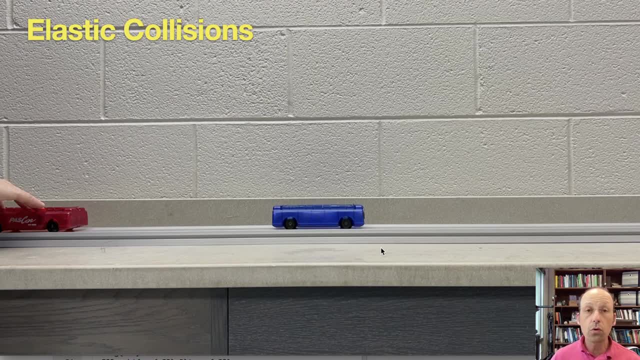 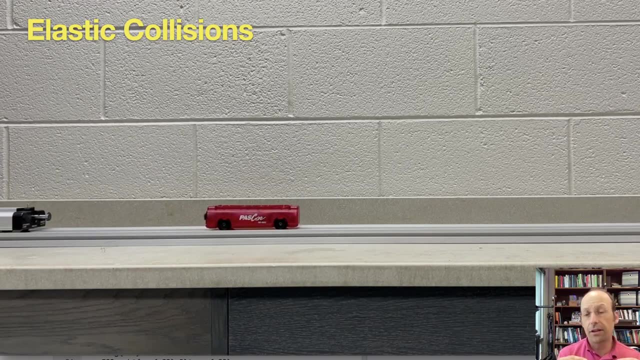 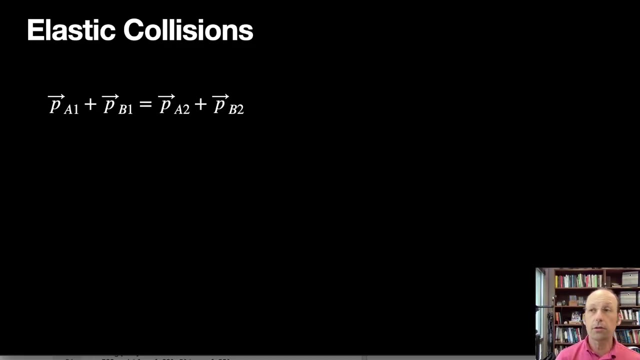 Let's use this in an elastic collision between two carts of equal mass. These are two carts. They have actually a magnetic bumper between them, So it looks like they don't interact, but they effectively do. And so here is my conservation momentum equation. 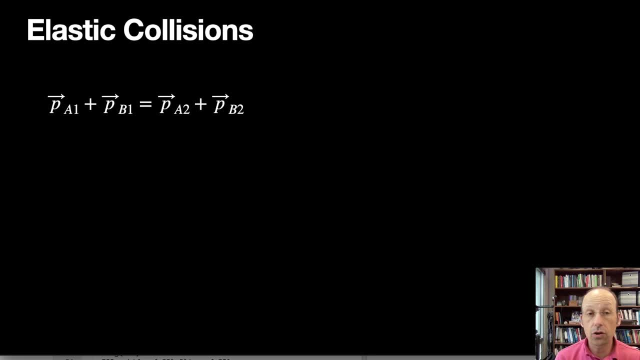 I already said that PA1 plus PB1 equals PA2 plus PB2.. And that says momentum is conserved. But for an elastic collision we also have this statement. This says that the kinetic energy of A before the collision plus the kinetic energy of B before the collision 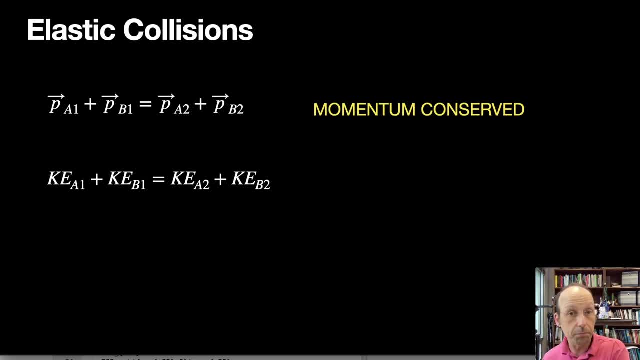 is equal to kinetic energy of A after plus B after, And we call that conservation of kinetic energy, And it's only true for elastic collisions. And of course we define kinetic energy as 1 half mv squared. Now I'd just like to point out here that v is a vector. 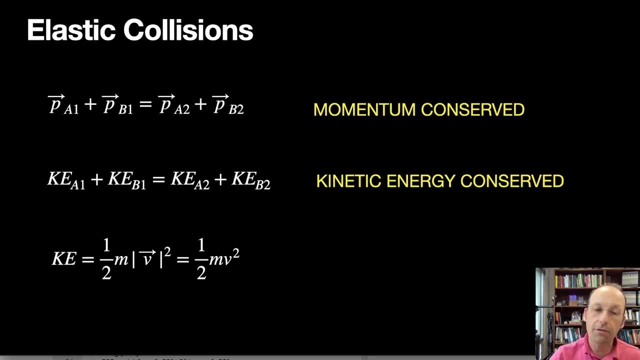 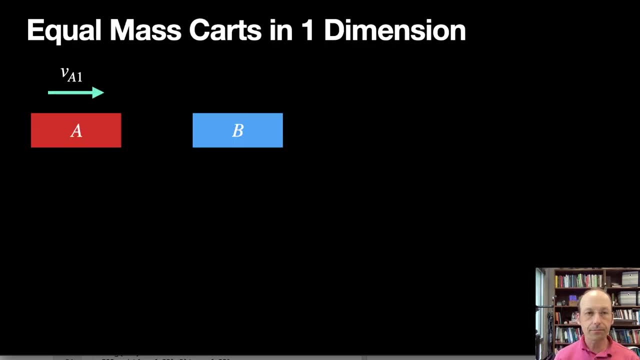 So, technically, what we do is we find the magnitude of that vector and then squared, But we'll always write that as v squared, because this word is too lazy. That's fine, It's fine, It's fine, right? Okay? So here are two carts in one dimension. 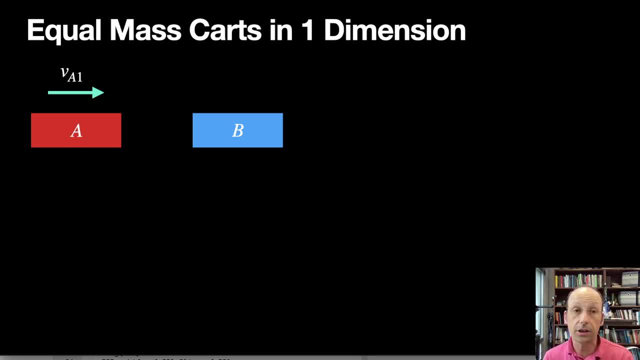 So I can just write these velocities as scalar values. They're in the x direction And I have car A coming towards car B and car B starts at rest And they're going to collide. So I'm using this bar to represent time, right. 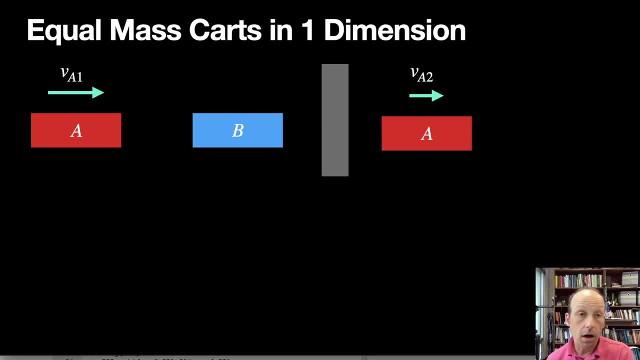 So now we're after the collision. So after the collision, car A has some velocity- vA2.. I don't know what it is, And car B has some velocity- I don't know what it is. We need to find out what those are. 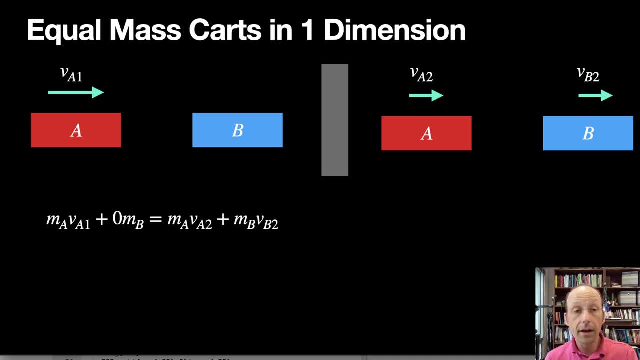 So this is my conservation momentum equation. So the momentum before mAvA1, car B has 0 velocity, so it's just 0 times mB, And then mAvA2 plus mBvB2.. For afterwards, My kinetic energy conservation equation says this: 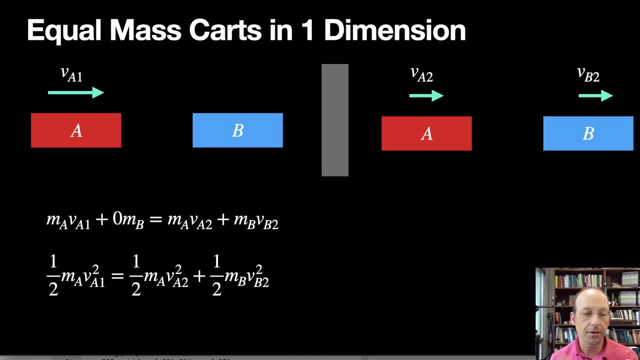 I left off the car B's kinetic energy because I was lazy. 1 half mAvA1 squared is 1 half mAvA2 squared plus 1 half mBvB2 squared, So the kinetic energy before is equal to the kinetic energy afterwards. 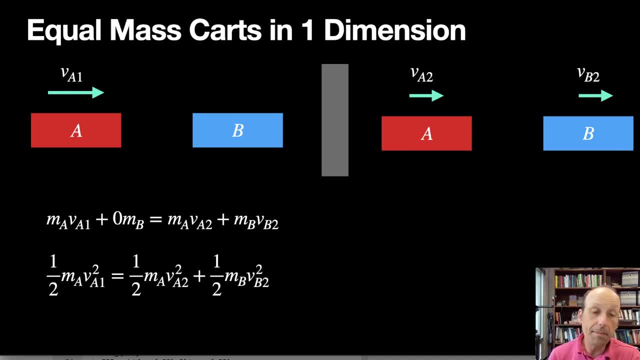 But I said that the masses were equal. So all these masses are the same. So all the masses are all the same. So that means that in that momentum equation I can get rid of the 0 and divide both sides by the mass. 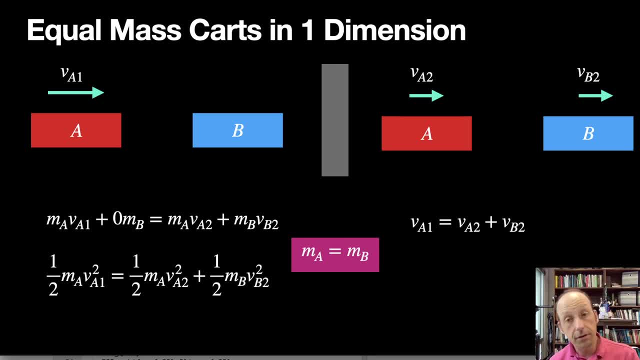 and I get a simpler equation: vA1 is equal to vA2 plus vB2.. I can do the same thing for the kinetic energy. The 1 halves cancel and the masses cancel, So I get vA1 squared equals vA2 squared plus vB2 squared. 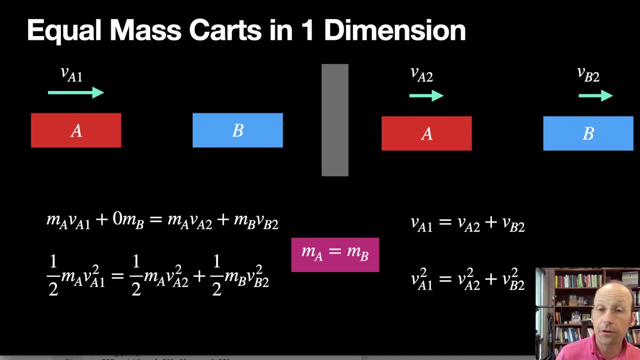 But again, I don't know vA2.. I don't know vB2.. And that's what I want to find. But that's the two equations I want to solve, for I have two equations, I have two unknowns. 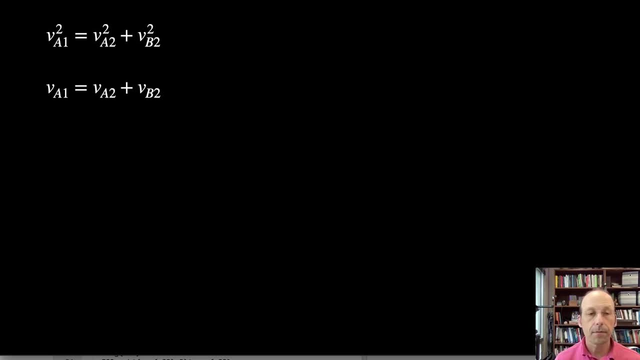 Let's get to it. So here are those two equations. I flipped the order just because. So the second one says vA1, and the first one says vA1 squared. So let's square both sides of the second equation. So if I do that I get vA2 squared plus the cross term twice. 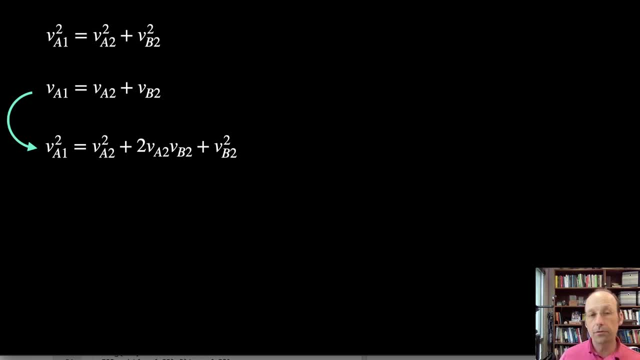 2AvA2vB2, and then vB2 squared, And then the first equation also has vA1 squared, So I can set those two equal to each other. So vA1 squared is vA2 squared plus vB2 squared. 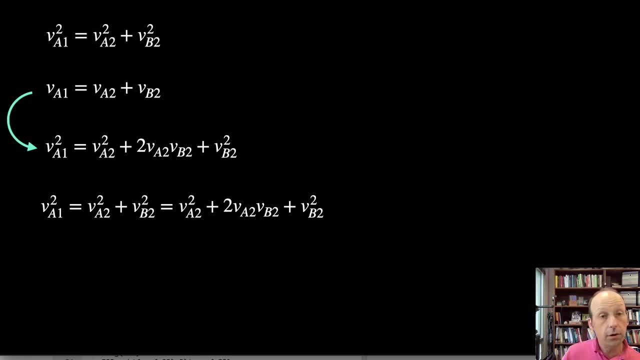 So I can set those two equal to each other. So vA1 squared is vA2 squared plus vB2 squared, But it's also equal to vA2 squared plus that cross term plus vB2 squared. Well, I can start canceling some stuff here. 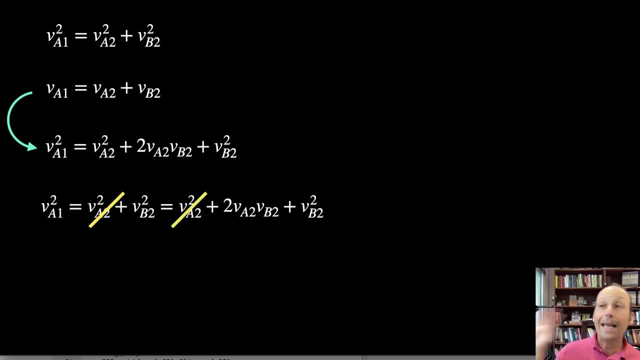 So there's vA2 squared. Here's vA2 squared Canceled. vB2 squared Canceled. So now I have this: 0, that's all that's left on the left hand side is 2vA2vB2.. 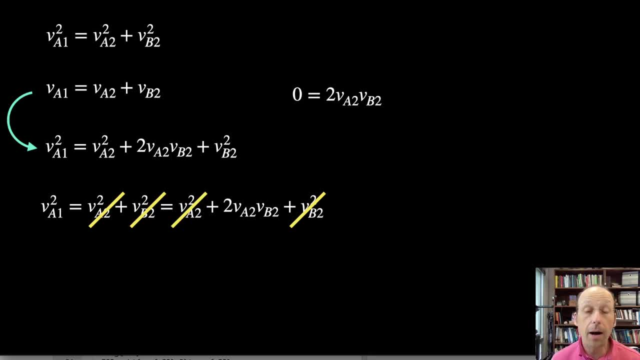 Okay, so that's my equation. That's what I'm stuck with. So there are a couple of options to solve this equation. solve this equation Number one. that's the equation I want to solve. I could say: VA2 is zero. If VA2 is zero, I multiply that by VB2.. I do indeed get zero. So that works. That's fine. 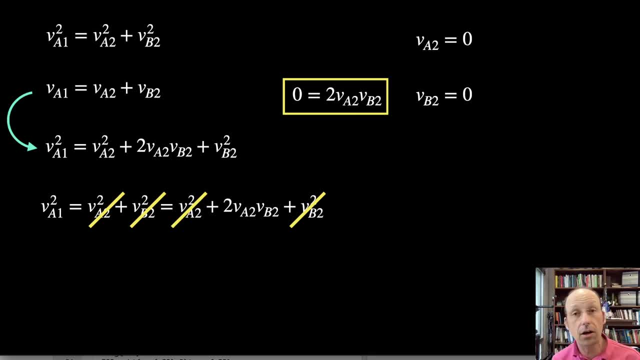 I could say VB2 is zero. That says the velocity of the second car is zero after the collision, And if I put that in there, algebraically it works. But that means that the target cart, the cart that was stationary, stayed stationary, It's stationary and then after it's still 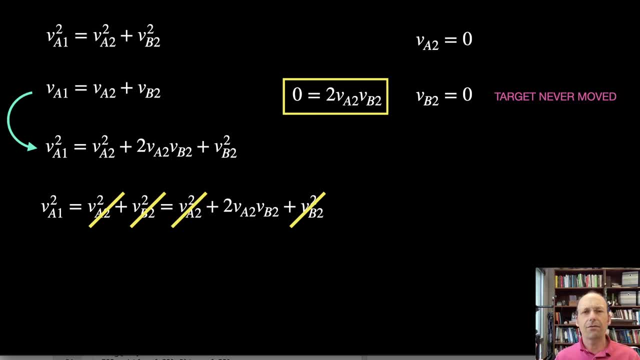 stationary And that's like it never even got hit. It works. It's a solution. It's just a boring solution. It's like the car missed. And then I also have this solution. I could say: what if VA2 and VB2 are zero? That works in this equation. But over here this equation says: 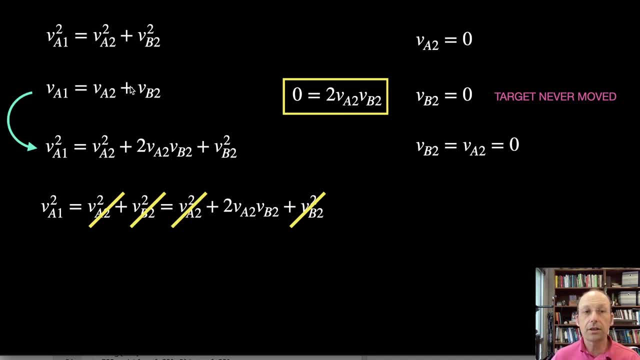 VA1, which I know is moving, has to be equal to some value, So those both can't be zero. It doesn't. the momentum is not conserved, if that's true, So I don't want to use that one. So that leaves me with this: VA2 is zero, And if I use that in my momentum equation, 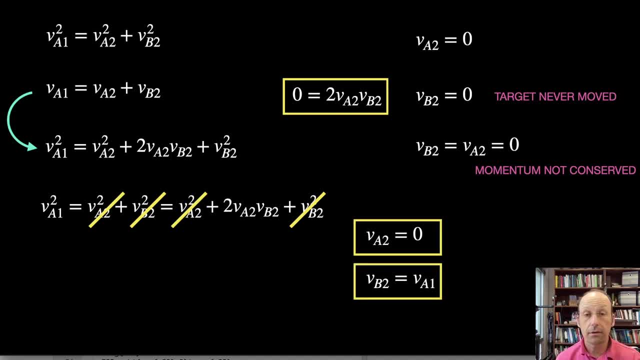 then VB2 has to be equal to VA1.. So that's what we have. So we have the car coming in, the launch cart stops, the target cart moves And you've seen that with the pool balls that happens. This happens with the elastic collision between two objects of equal mass. It has to be: 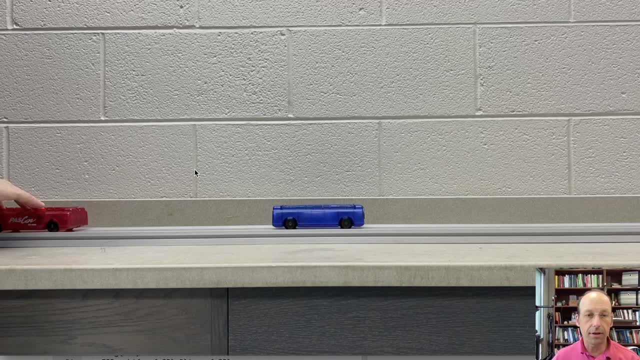 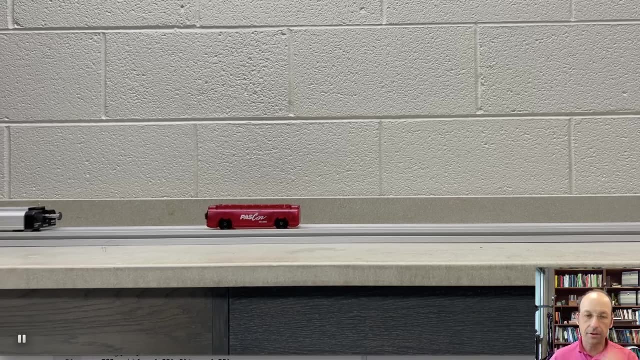 equal mass. And so here- we already saw this, but here it is again. So the red car stops and the blue car moves, And it moved a little bit. It wasn't a perfect collision, but that's fine, Okay. And that other cart. I was just using this other cart over here. 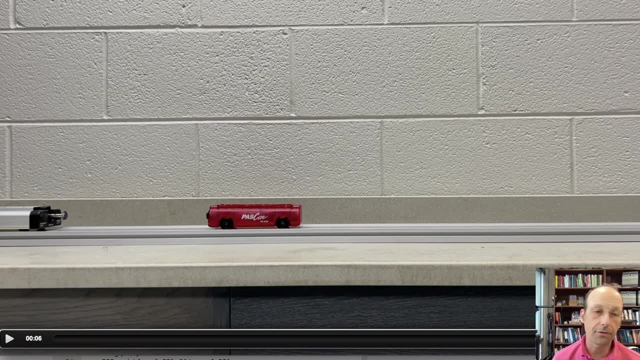 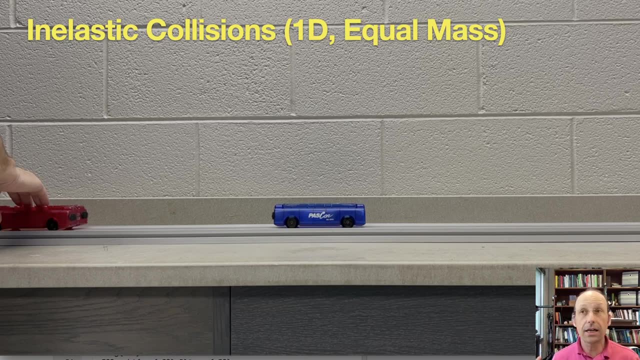 to launch the red cart. I tried to launch them all the same way, but that's fine. What about an inelastic collision? So in an inelastic collision, kinetic energy is not conserved, But what happens is the two cars stick together. So if the two cars stick together, then what would their velocities? 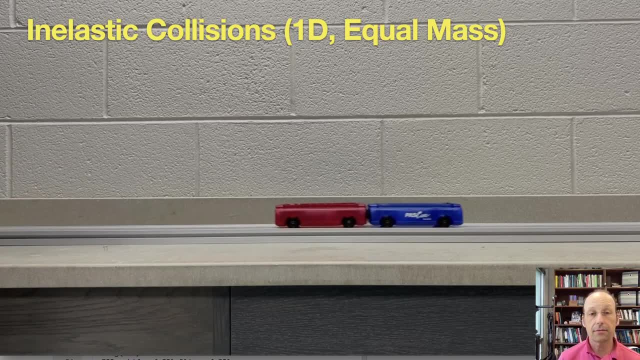 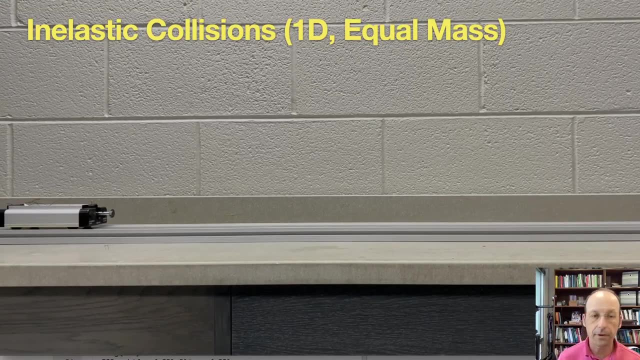 be afterwards, So let's do this. That's an inelastic collision. They stuck together And those two cars have Velcro things on them, So when they hit they can stick together. You just have to flip them around. So here's our two cars. 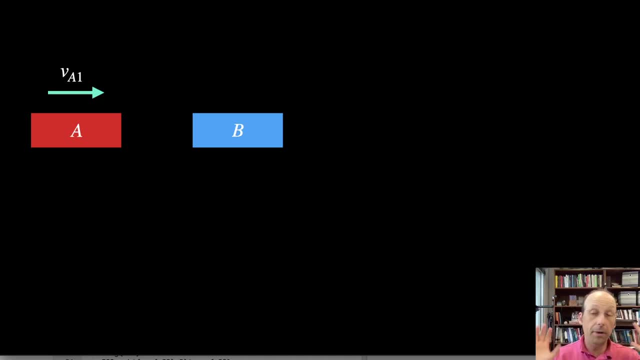 beforehand It looks the same before the collision: Car A and Car B, they're the same mass, And that's my little bar, for stuff happens And then they stick together. So the key thing here is that VA2 and VB2 are the same. So let's write down our conservation of momentum equation So, MA. 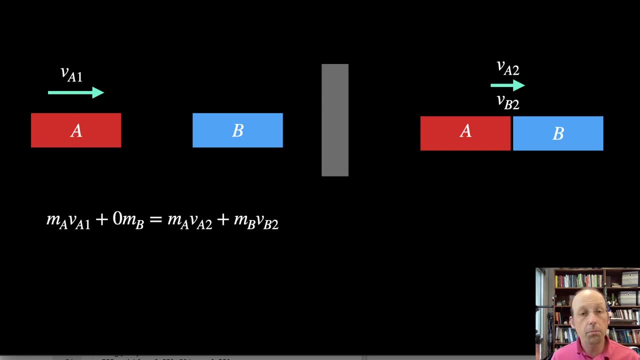 VA1, plus 0, same as before is MA, VA2, plus MB VB2.. Again, the masses are the same, So the masses cancel. So I get VA1 equals VA2 plus VB2.. That's the same as I had before, But now I have. 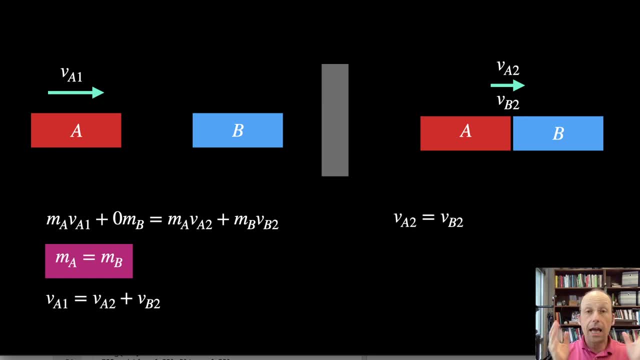 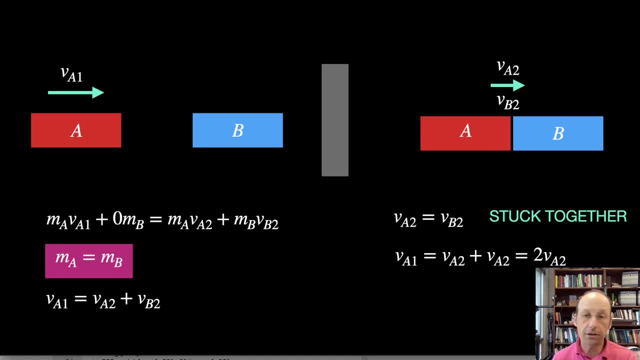 plus VA2, or 2VA2.. And if I solve that for VA2, I get: VA2 is equal to one half the initial velocity And that's also VB2.. We already said they're the same, So the two cars come together. 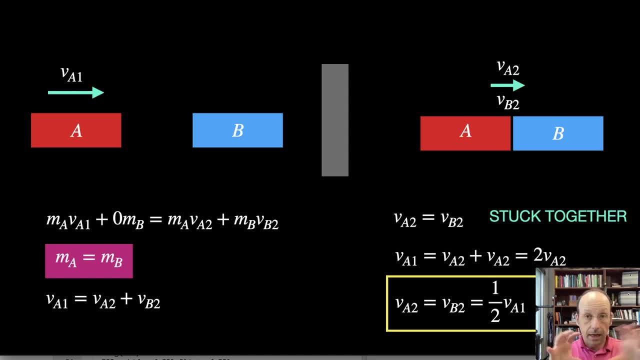 they stick together- I put a box around this because it's important- And they move at half the speed, But that's only if the two cars start with the same mass. This is a special case. Okay, what about something that's not elastic and not inelastic? So remember elastic. 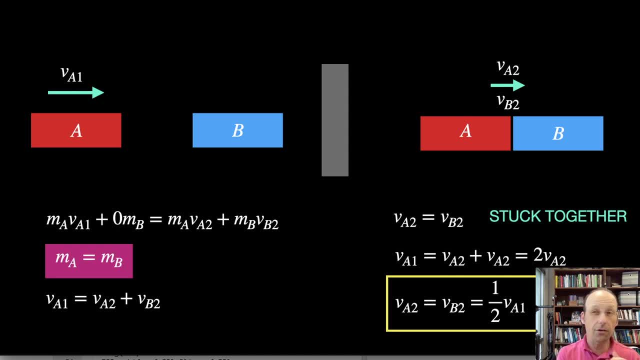 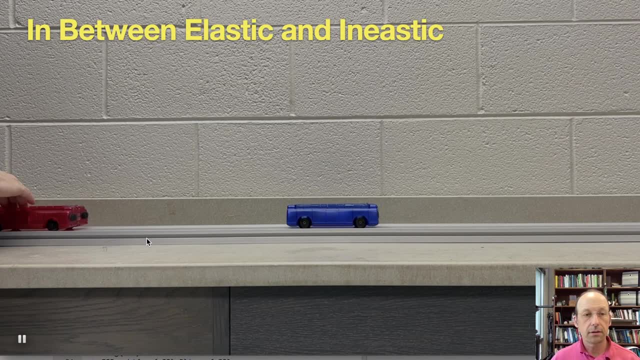 kinetic energy is conserved. Inelastic. they stick together, But it's possible to make a collision. that's neither of those two, And this is what that would look like. So here's my two carts. Now they're going to hit And you'll notice the red cart doesn't stop right, It continues. 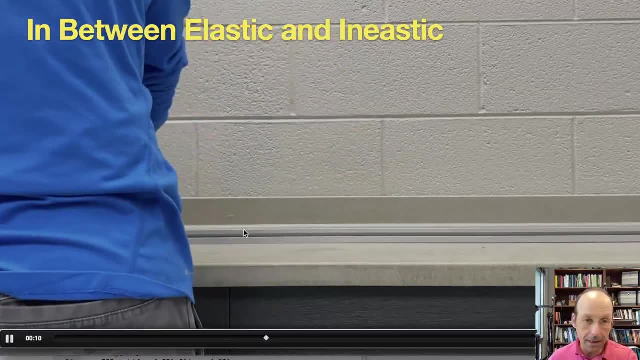 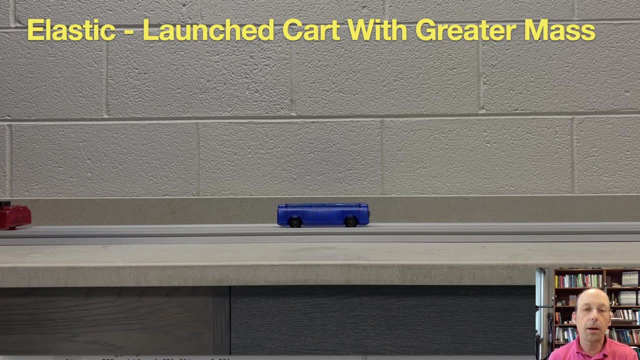 moving forward too, And the little creeper car comes into. and there's me, because I'm resetting things because I didn't turn the video and you don't need to see that. Okay, what if they don't have the same mass? I'm going to show you a couple examples here. What if they don't have the same? 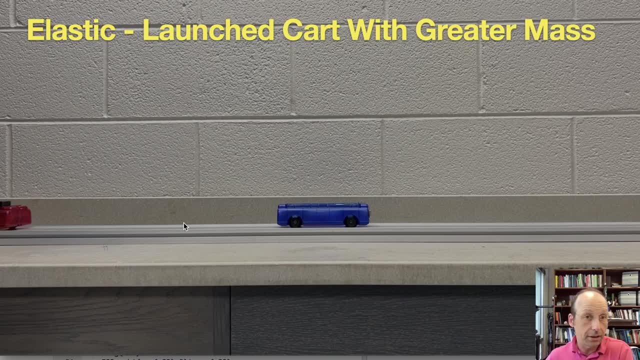 mass. Again, it doesn't work where the red cart just stops. This is an elastic collision where the launch cart has extra mass. You can kind of see it right there. Extra bars on that mass And boom, Now it doesn't stop. They both move the other way. The blue car actually moves a lot faster. 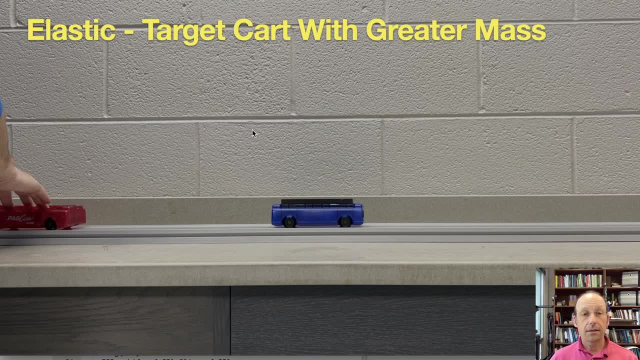 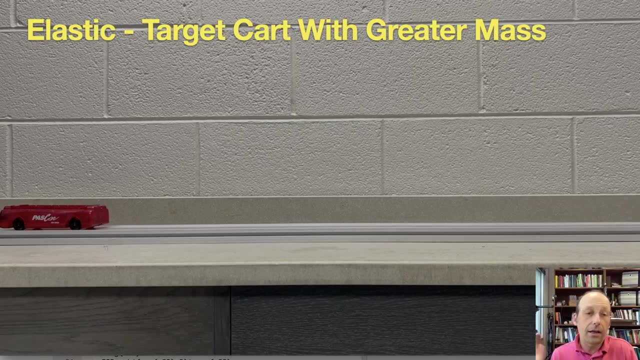 What if the target cart has extra mass? Again, we don't get that same situation. Kinetic energy is conserved, But that's that. So I'm not going to solve all those problems. I'm just showing you what happens if you change the mass. 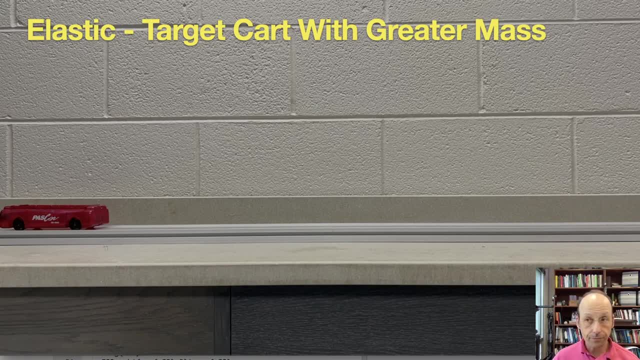 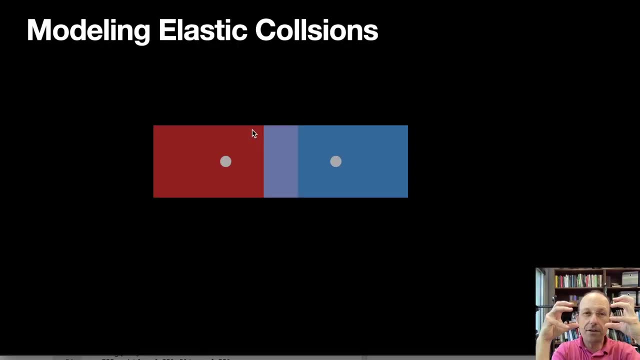 I'm going to show you what I see on the screen. I don't have extra mass, And this is how it looks in real life, So you can see what's happening here. I'm going to say that if you pull this button, then I'm going to say that I have the same mass as the main car. Then I'm going to say that: 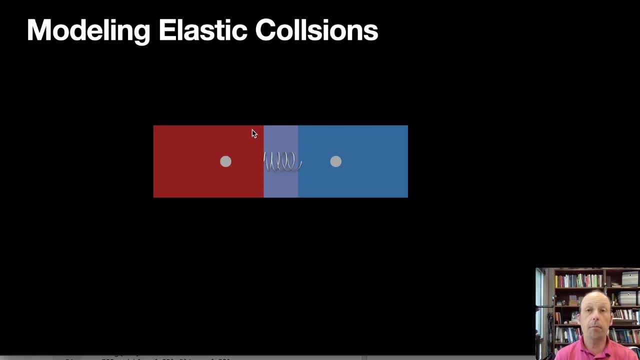 it's not the same thing. if you pull this button, then it's going to say that they overlap, And that's how I'm going to create a model for this. Okay, so imagine that I have these two cars. Here's my red and my blue car. Imagine that they overlap a little bit, and when they overlap, I can. 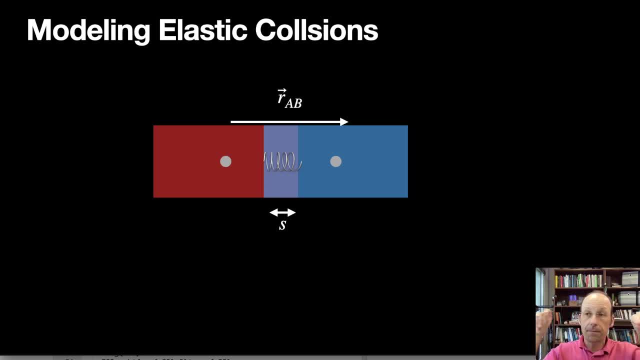 say that there is a spring pushing them apart. That's not crazy, That's kind of true. And if I do that, I can say that this overlap distance is s, and I want to find that. So I'm going to model this. I'm going to have the center of the two carts as the position of the 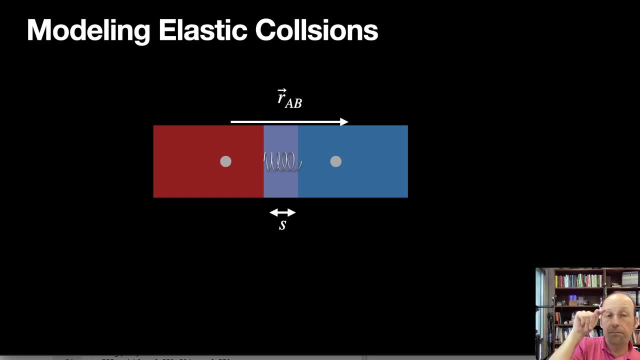 carts. So this vector, RAB, is important. It's the distance, it's the vector from the middle of A to the middle of B, And then I have the length of the cart. So I want a relationship between the length of the cart and RAB, defined S, And so you can see here if they're compressing a spring B is going. 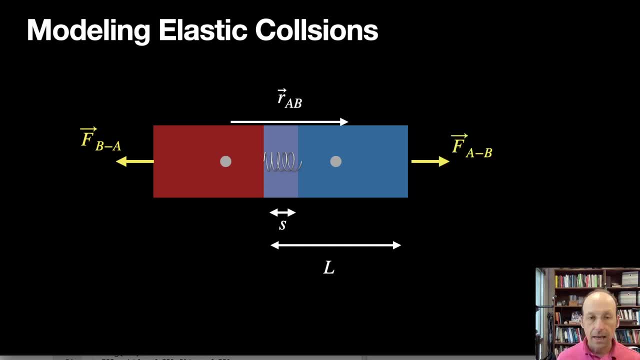 to push on A that way, A is going to push on B that way, And I can write the following expression for the magnitude of those two forces. It's going to be the K, the spring constant times, the compression S, And that compression S is the magnitude of RA minus the length. L Is that? 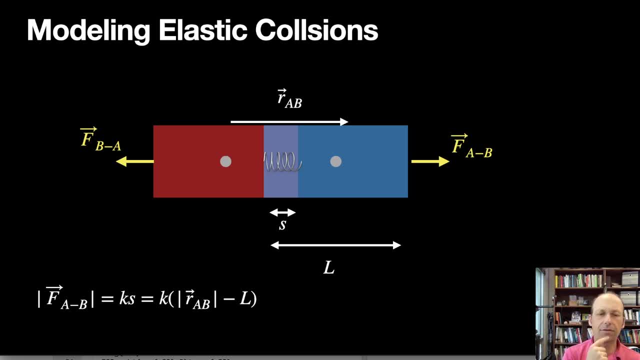 backwards. It's actually backwards. I think that'd be backwards. You'd get a negative sign there. but it's okay because I said magnitude right, So I didn't cheat. But the problem is that, as that compression S is going to be the magnitude of the cart, it's going to be the magnitude of the. 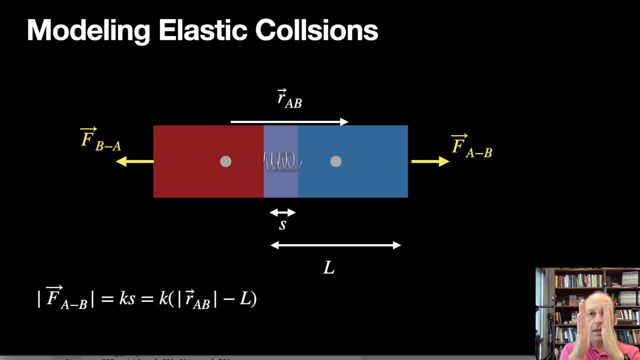 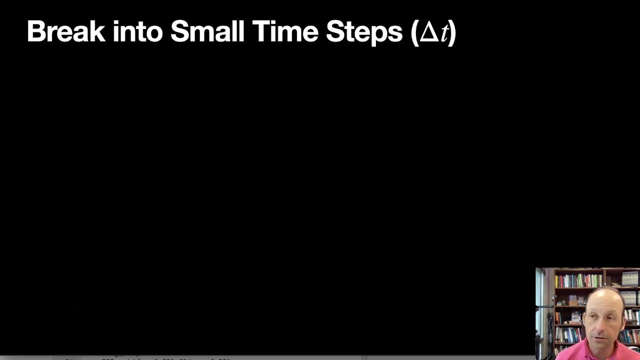 spring And if it compresses, then they're going to have a force and it's going to keep moving and the force is going to change. So I have a non-constant force. How do we deal with situations with non-constant force? And the answer is to break them up into small time steps. 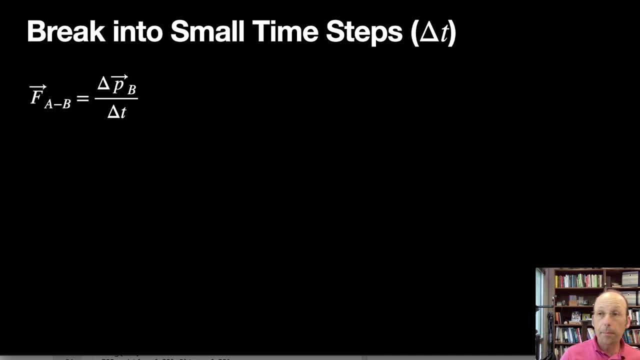 So let's say I look at the forces on car B. This is the momentum principle for car B And if I can write the change in momentum for B as PB2, which is hard to say, PB2 minus PB1.. So PB2 is the momentum principle for car B And if I can write the change in momentum for B as PB2,. 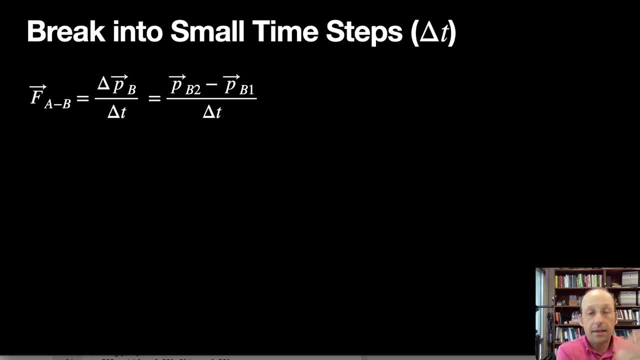 is the momentum of the car after some time step at the end of the time step, not the collision, And PB1 is at the beginning of the time step. So the difference in those momentums is my delta P. Now if delta T is really small, I can assume that this force is constant. It's totally not. 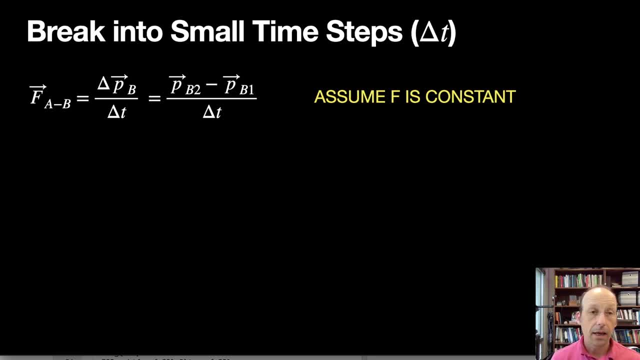 constant. Okay, I'm just making that assumption that it is so that I can do this problem And if I do that I can solve for PB2.. PB2 is the initial momentum, PB1, plus that force times delta T And we call this the update momentum step. I'm going to update the 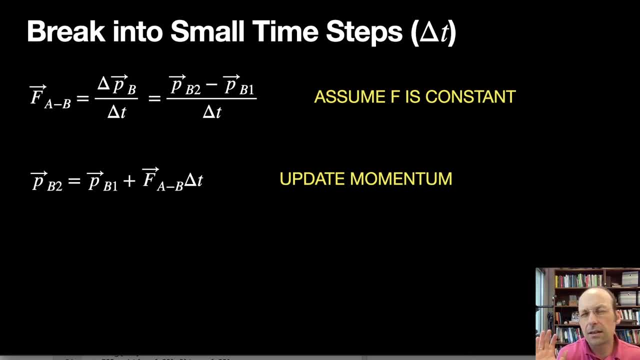 momentum over that short time interval, And then delta T, let's say it's one one thousandth of a second. Okay, Now I can also define the velocity as the change in position. So I'm using R for position, RB is the vector position of car B, The velocity is the change in position over time, And 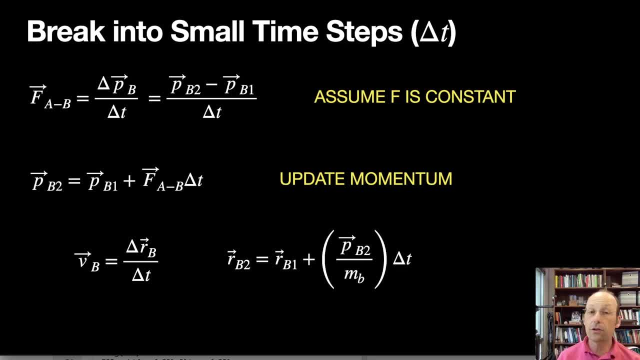 again, I'm going to assume that it's constant, even though it's not. And I can do a similar thing to find the position of the car at the end of the time step. So I'm going to use R for position. The end of the time interval, RB2.. And it depends on the velocity which I wrote as the momentum. 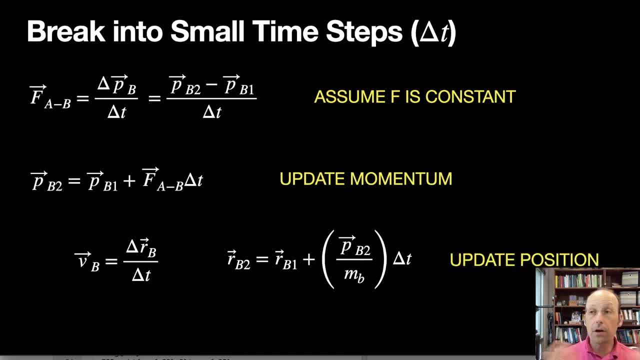 divided by the mass, multiplied by delta T, And we call this update position. Okay, So I just need to redo this for car A, because I have two cars. They both have forces acting on them And since I want to do it, let's say for a second: and delta T is one, one thousandth, that's a thousand times. 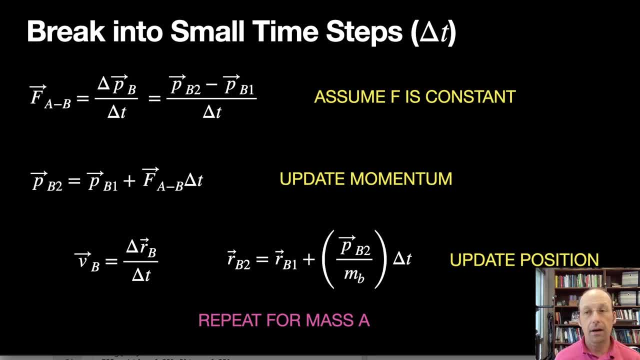 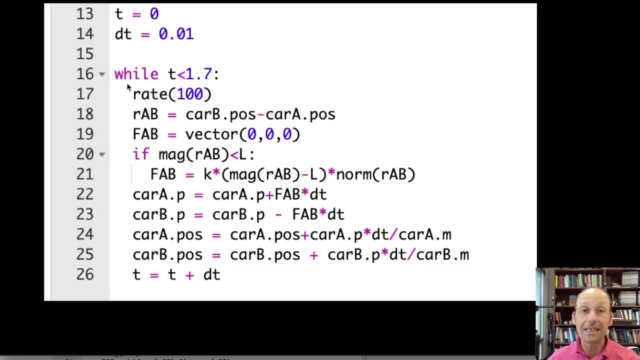 for both cars. So that's two thousand Steps, And I don't want to do that. No one wants to do that, But Python will do that, Okay. So here's a Python program that does exactly that. This is part of the program I didn't show you. 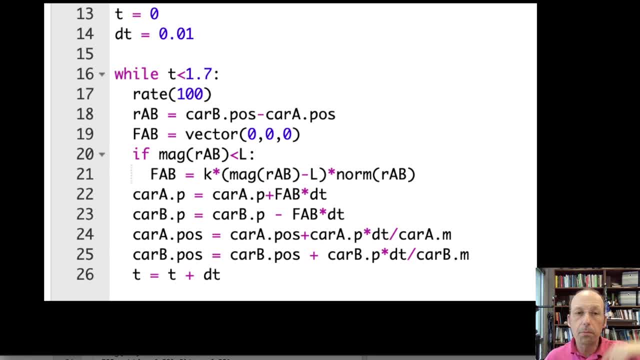 everything, But I'm going to show you how it runs. So this is a loop going over time. I have a time step of just one, one hundredth of a second point, zero one. So here in line 18,, RAB is the vector. 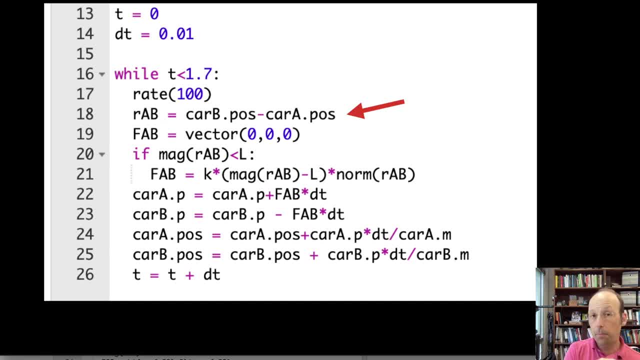 from car A to car B. So it's car B minus car A to car B, And I'm going to show you how it runs. Okay, That's that vector, That's that vector R, And I want to see if that vector shows that. 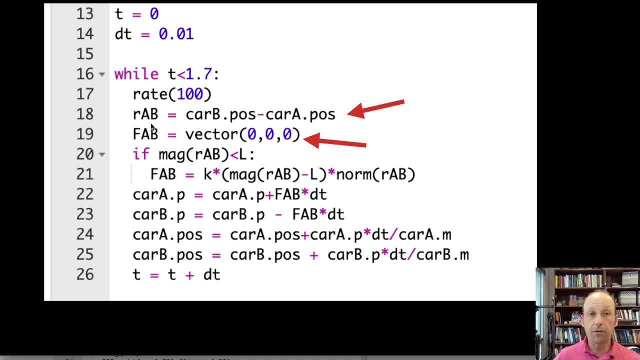 they're overlapping. If they're not overlapping, I want the force to be zero. So every time I go through, I'm going to set the force as equal to zero- the force of car A on B- And then, if it's not, if they're overlapping, I'm going to change it to this, which is the value of the force due. 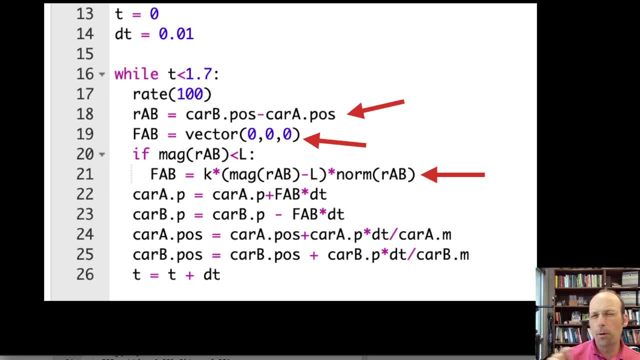 to the spring. So I have that compression minus the length And that norm. RAB is just a unit vector So I can get a vector value for FAB And then in line B I'm going to set the force to 22.. I update the momentum for car A. update the momentum for car B. 24 and 25 updates the. 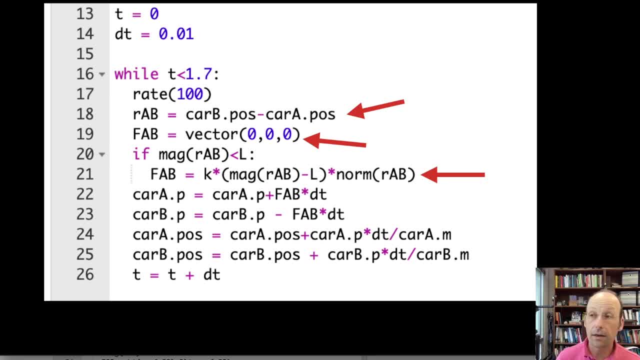 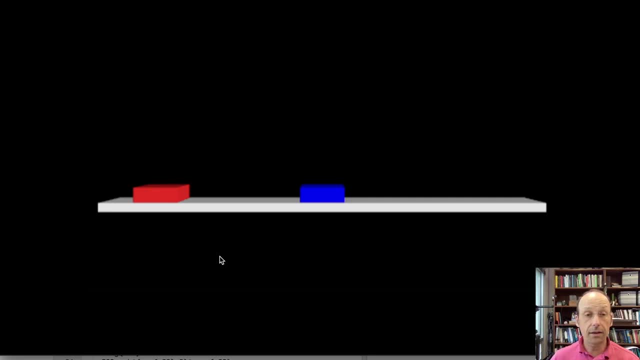 positions and then update time, And you just keep doing that over and over again And it works. I'm using WebVPython, So WebVPython has these three-dimensional tools to make three-dimensional animations, which is super awesome, And this is what it looks like. So there's my two cars. 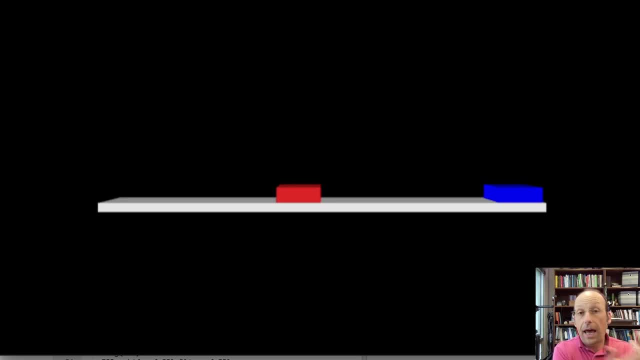 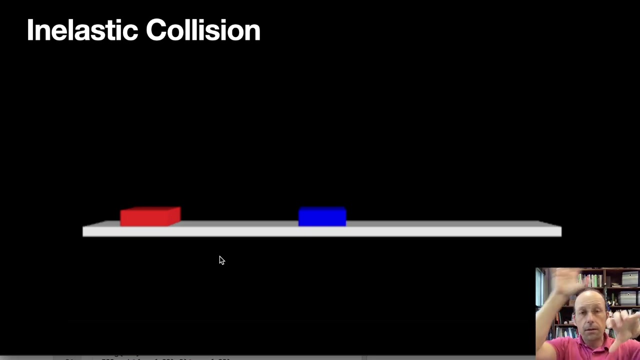 And the cool thing is that I can reproduce. I can reproduce what actually happened, but by breaking it in small steps and doing this, update momentum, update position- And you can see that it does indeed work. What if I want an inelastic collision? How do I model that with forces? Well, in the previous 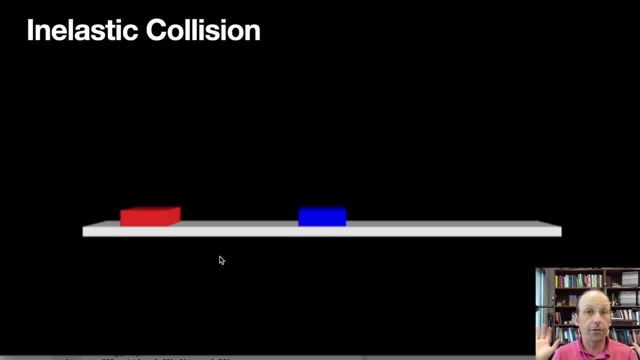 collision. once they stopped overlapping, there's no force. The only difference here is once they come in contact, the force is always there. So if it leaves, they're no longer in contact. there's still a force pulling them back together. So you'll see here that I 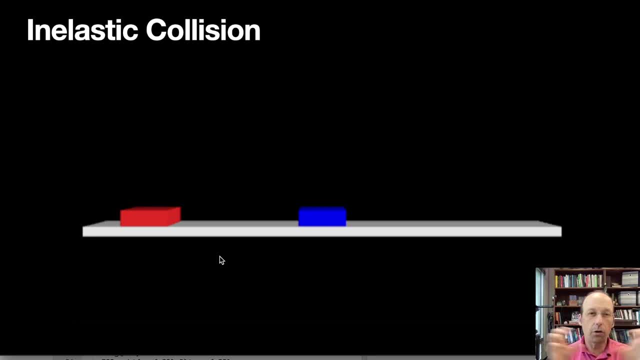 I had to increase the spring constant, but there's a little bit of shaking in order to make them stay together. but it mostly works And they move away with the velocity of half the initial velocity, So it still works. What about an in-between collision, In this case? 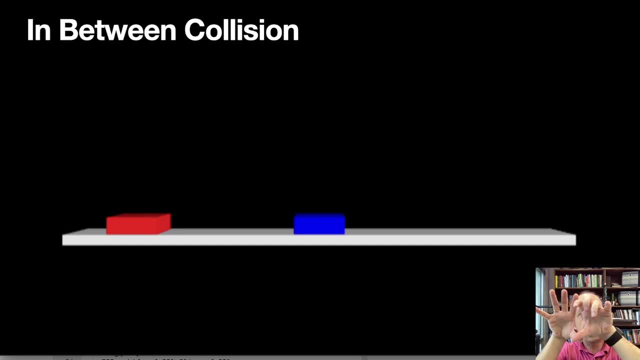 the trick here is to say the spring constant for when they're colliding is greater than the spring constant pushing them apart, So that that work done by the spring when it pushes it out isn't as great as the work done on the cart to compress it. So you lose energy. 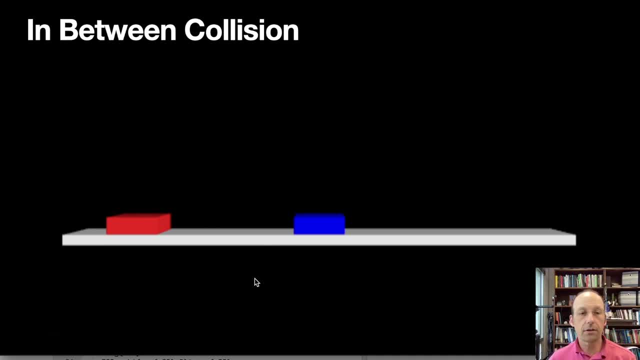 and you get a lot of force. So that's the trick here. And then the trick here is to say the spring constant for when they're colliding and you get a just a normal collision And you'll see that that red car doesn't stop. Okay, Now I can use this for Newton's cradle, because that's where 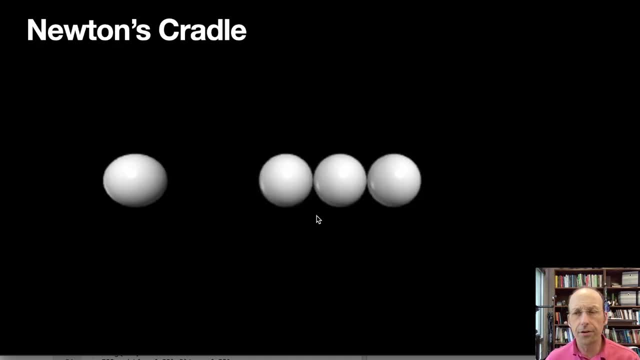 I started with Newton's cradle. I only used three balls here because I got lazy. I didn't want to draw. I think that the the, the video above, has five balls, but it doesn't really matter. So what's going to happen here? This is just like a car, except that now I'm using the radius of. 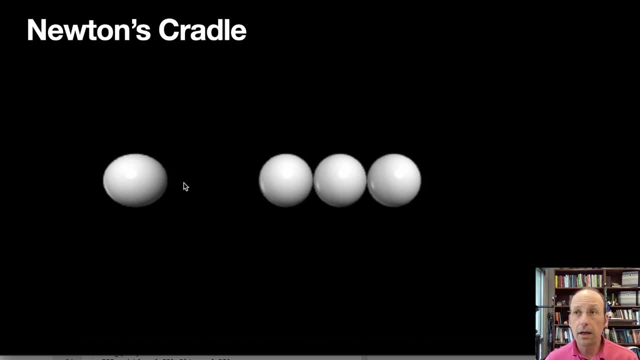 the ball to see if they overlap. And so I'm going to make a force between this first ball, that's, and that ball if they overlap, And then there'll be a force between this ball and that one if they overlap, and this one and that one overlap. And they do overlap, Okay, Because it's not a perfect. 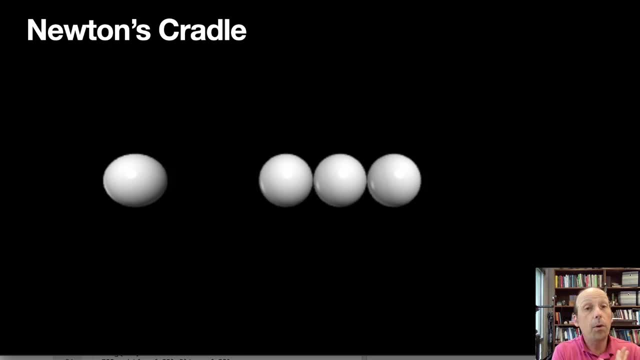 model. I wanted to make it be able to be seen And we want to see: does it work? Does it shoot that last ball out and the other one stop, And each collision should do that. So overall it should do that too, And it works right When you build a model for something real. 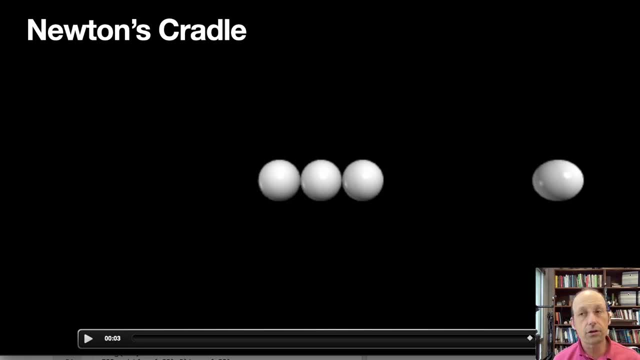 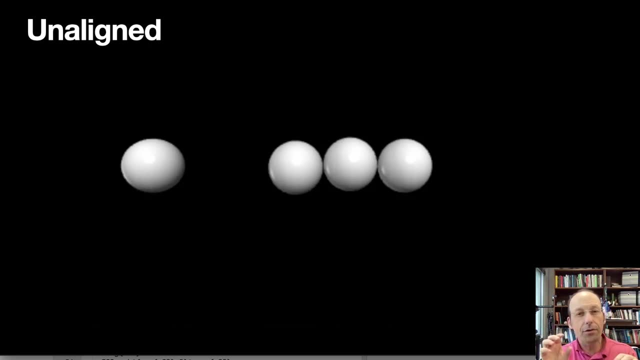 and you get, you can reproduce it, then that's a good sign that you're they understand what's going on. Now, just for fun, I can do something like this where you it may be difficult to see, but all those balls, the three balls, aren't completely in a straight. 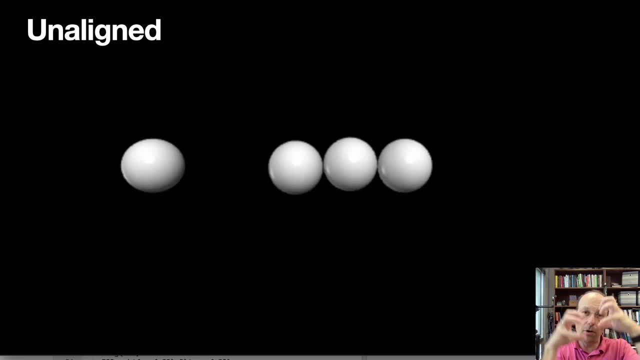 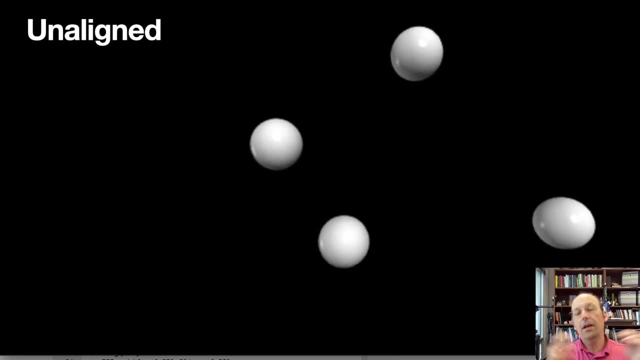 line And now when those forces interact, they're going to push them off, off axis a little bit and it's not going to work as well. So let's run this one, You see now in a real nudes cradle. 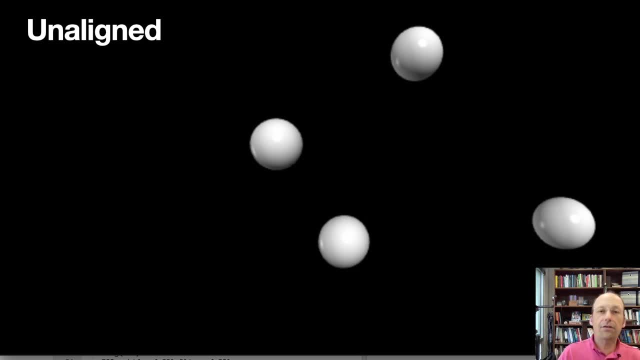 they'd be attached by strings. but just to show you that we don't get the same effect if it's not completely lined up. Uh, and that program is no different Then the previous one, except that the positions of the balls are just shifted off a little bit. 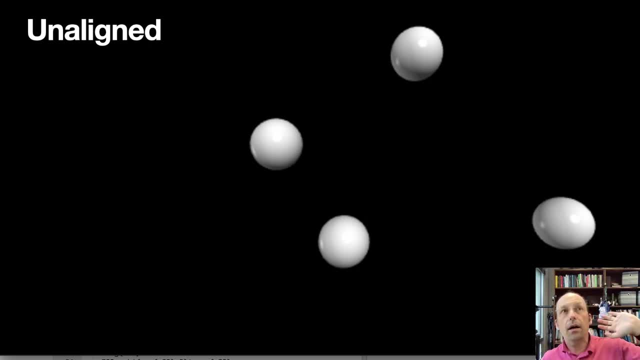 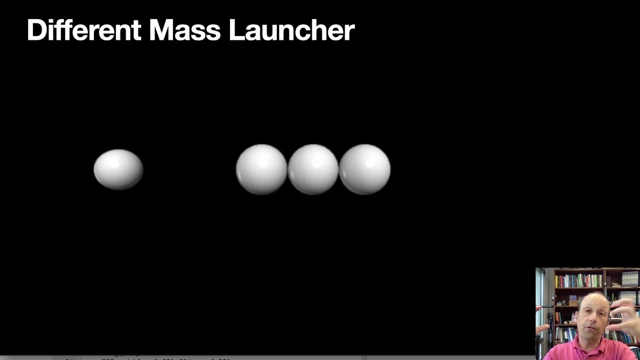 That's the only difference. Now, I did this for um, a video with the slow-mo guy shooting a smaller mass ball at a Newton's cradle, And so what would happen if I have a slightly smaller mass ball over here, Remember, in order for that situation where the launch cart stops. 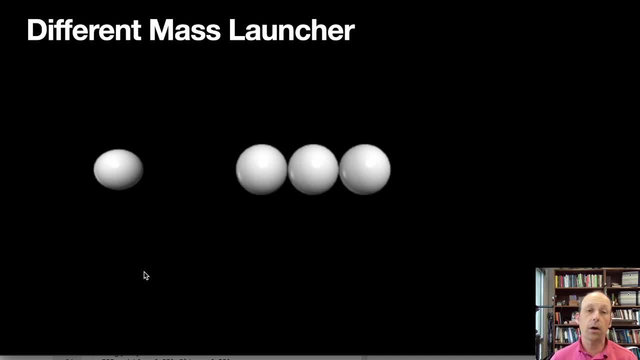 and other ones moves, they have to be the same mass. So if they're not the same mass, it doesn't quite work. And you'll see there it does. It doesn't doesn't quite work, Okay. So, but again, if you can model this and you really 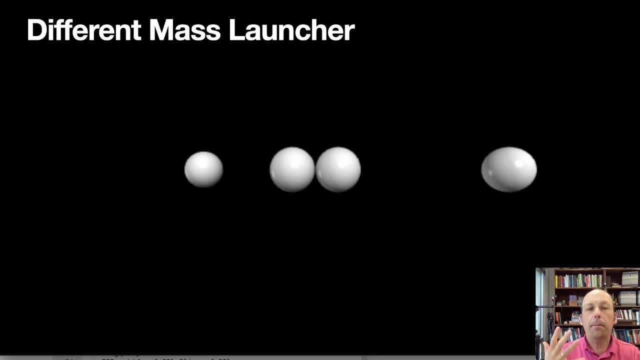 understand it and and there's just an introduction to these collisions. I'll make a better video later going over the details of how to make that Newton's cradle in Python, But hopefully that gives you a little sense of collisions, especially collisions in one dimension: elastic, inelastic. and in between, I'll talk to you later.